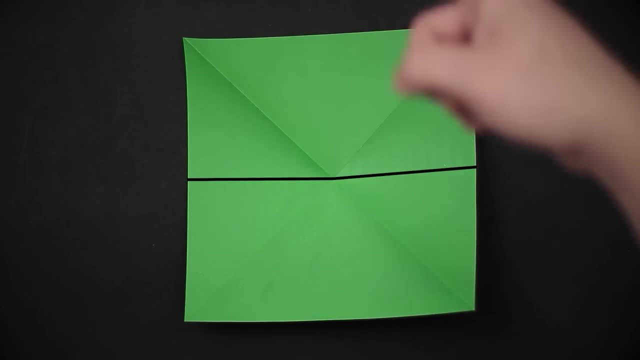 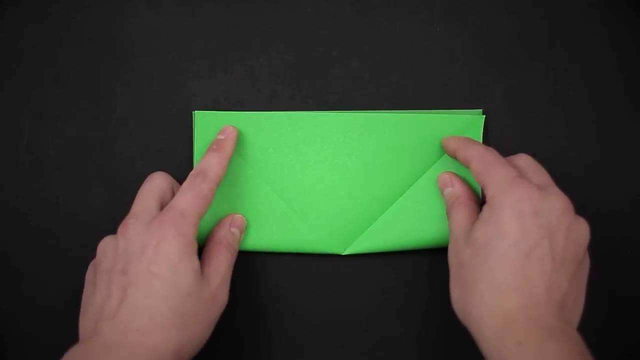 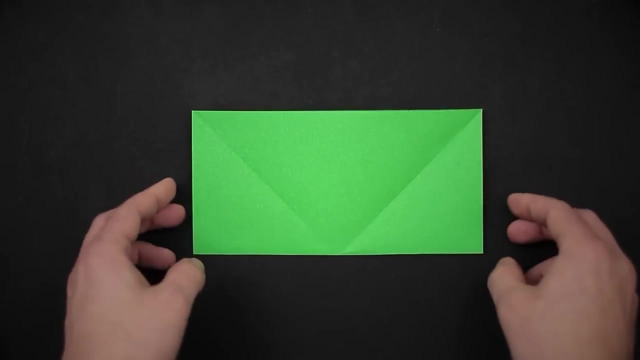 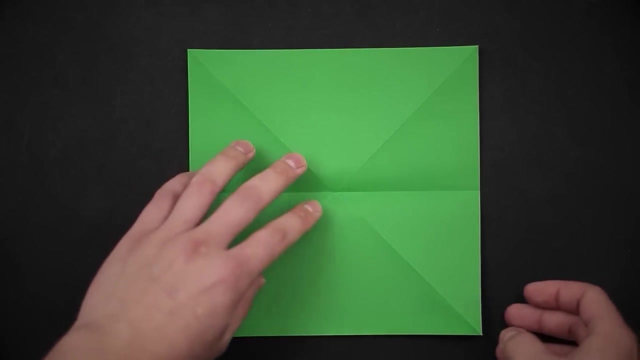 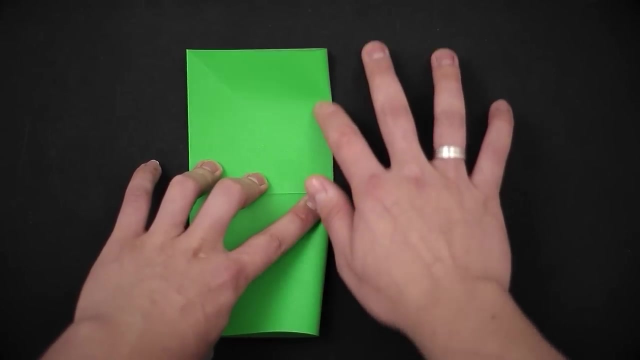 and fold it in half horizontally, And then we fold it in half vertically. We'll bring the bottom side to the top, Unfold it. And now for the vertical. let's bring the right side to the left, And here you'll see the center of the paper. 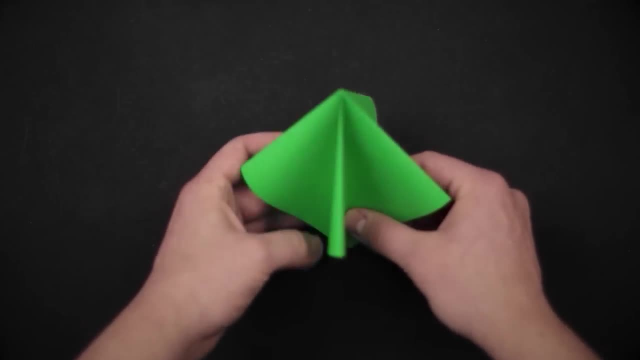 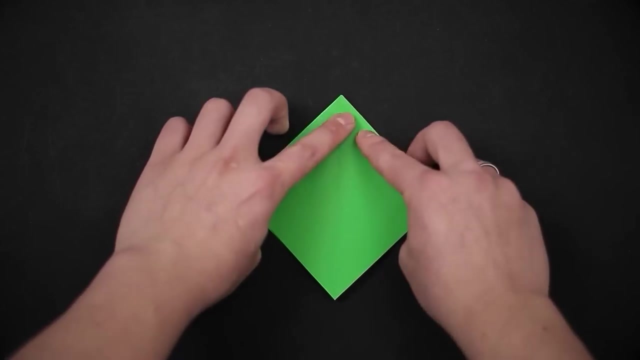 Having these marks ready, we can turn the paper over and push the four corners towards the center, closing it like this. Now let's keep the paper in the same position, with the open side down and reinforced it. very well, Now we're starting with the right side. 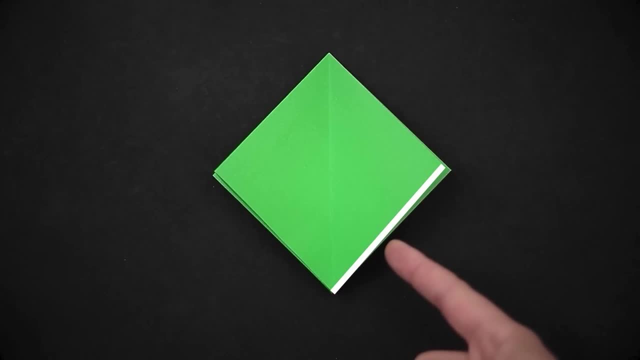 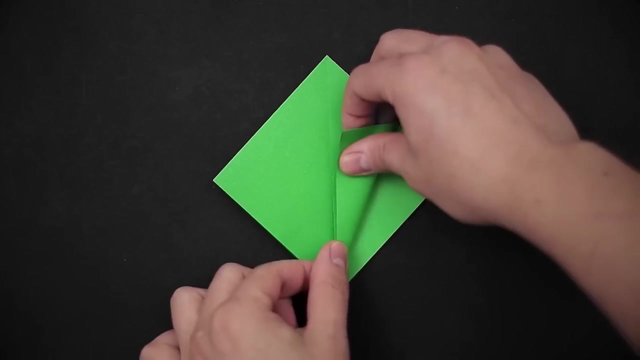 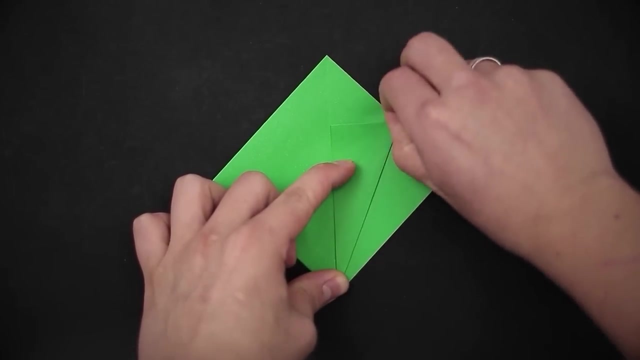 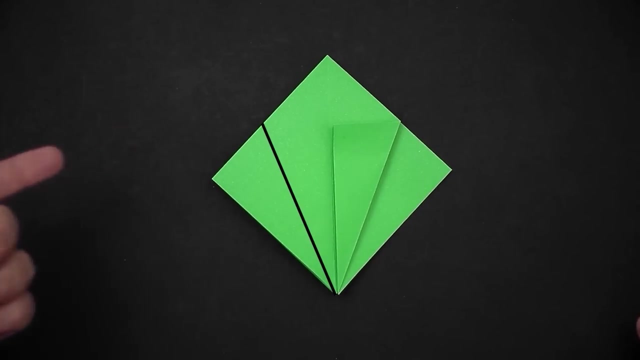 Let's take the lower diagonal edge of the first layer and bring it to the middle, making a new diagonal fold. So we just need to bring it carefully, aligning everything as perfectly as possible, And then we make a crease. Having done that with the right side, we can repeat the same thing with the left. 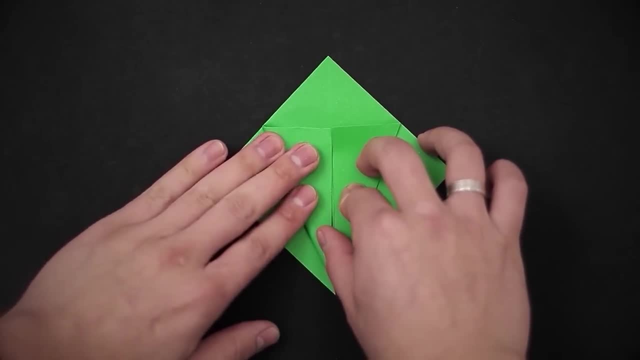 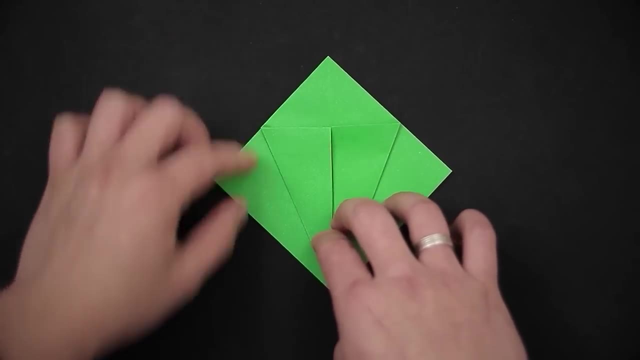 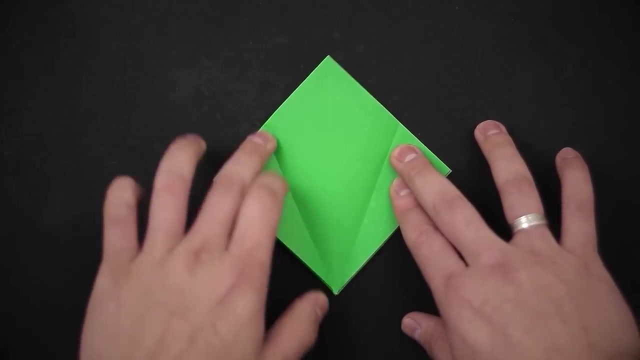 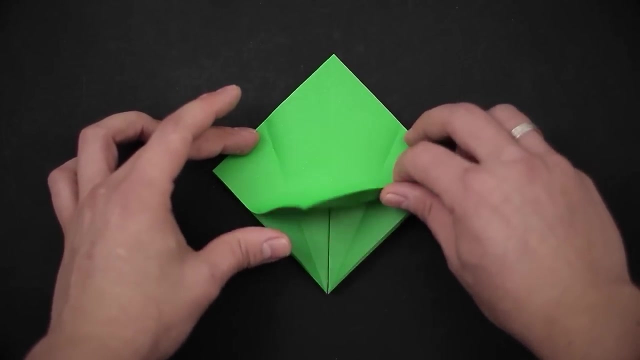 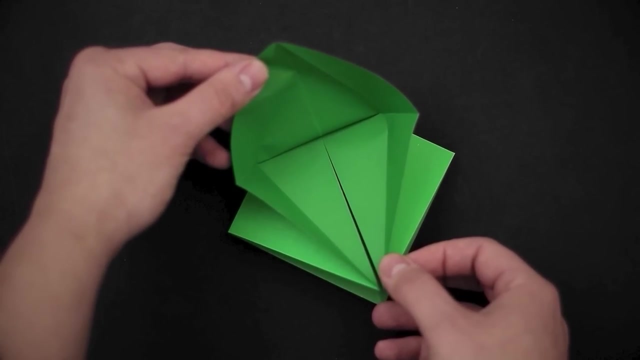 So just bring the edge to the middle And reinforce. Now we can unfold both. Okay, And for the next step we're going to have to open the first layer like this, And then, using the lines we just made, we're going to bring both sides to the middle. 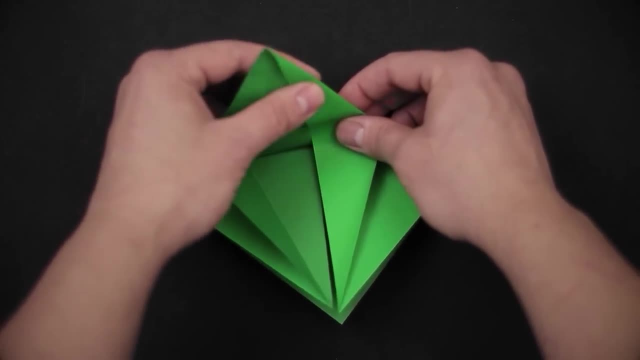 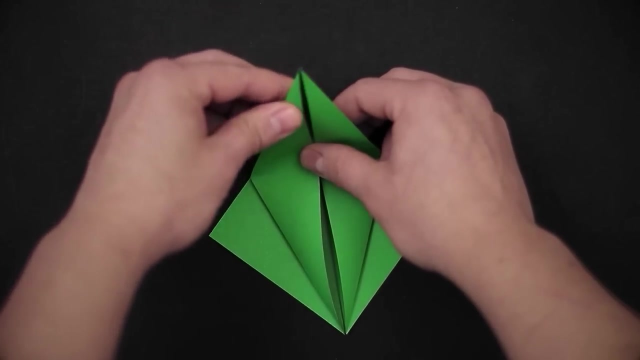 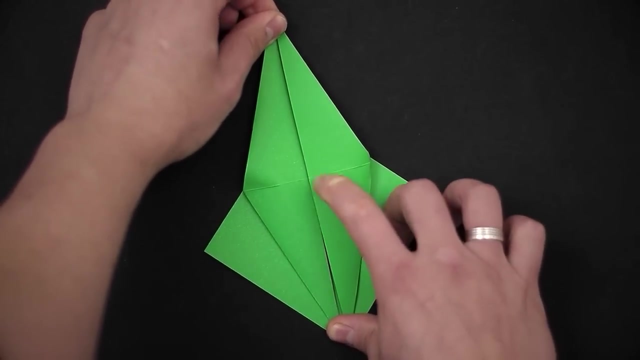 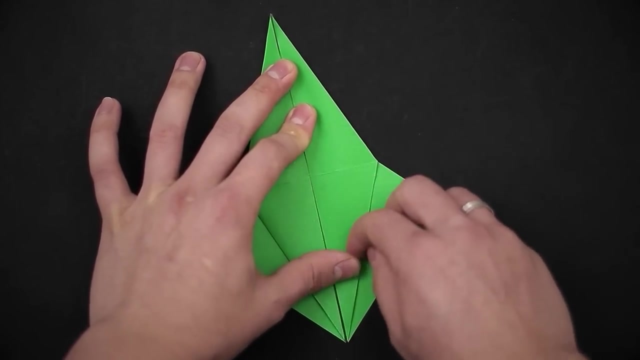 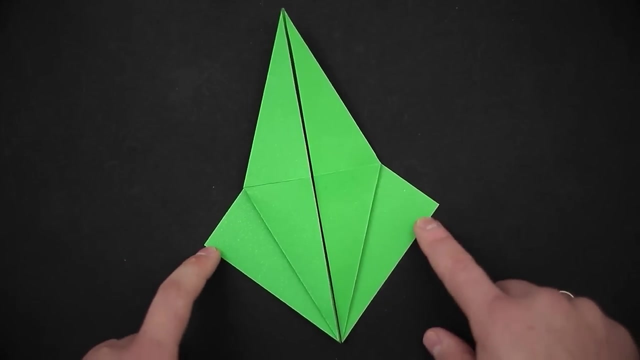 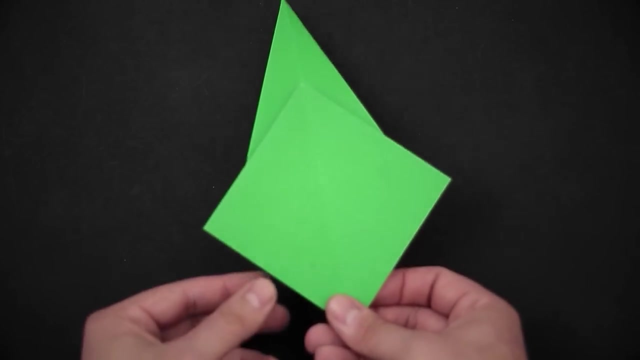 First the right And then the left, Okay, And then the left. Let's try to align everything very well, reinforcing what's necessary. And we have a new flap. Now let's turn it over And repeat the same thing with this side. 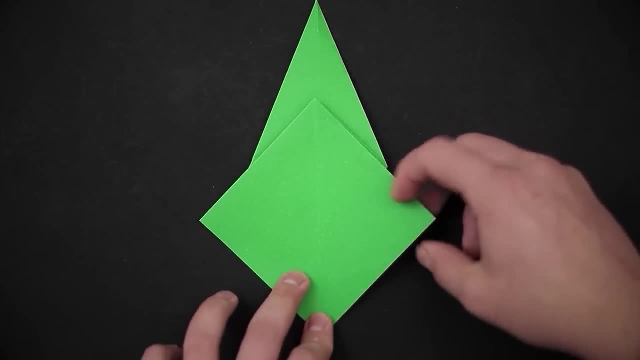 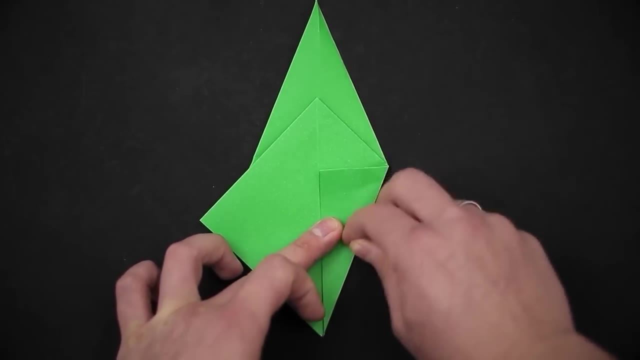 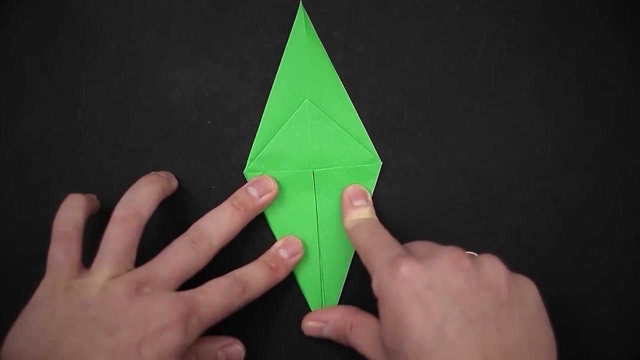 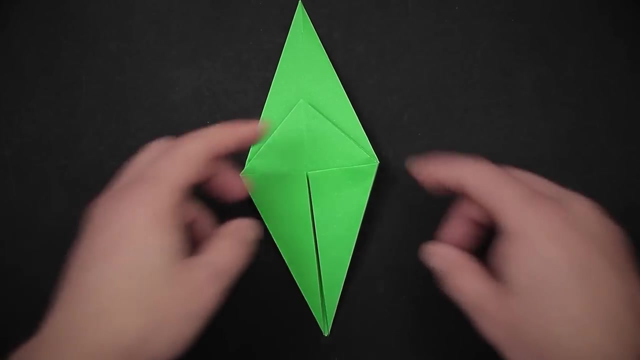 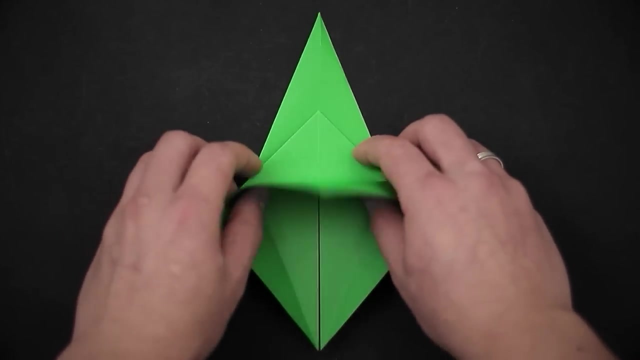 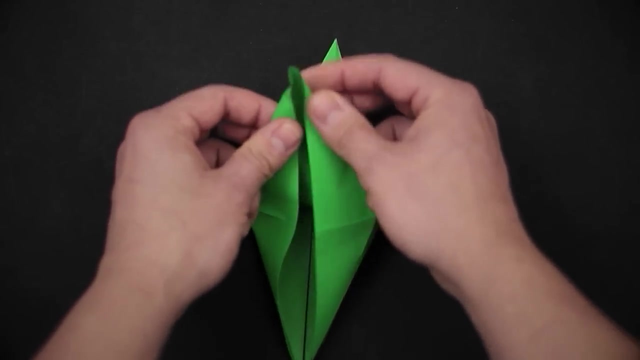 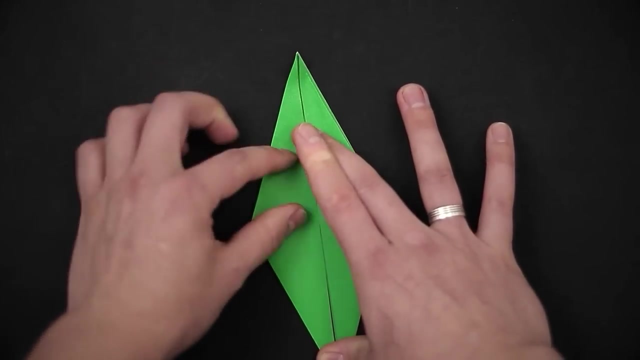 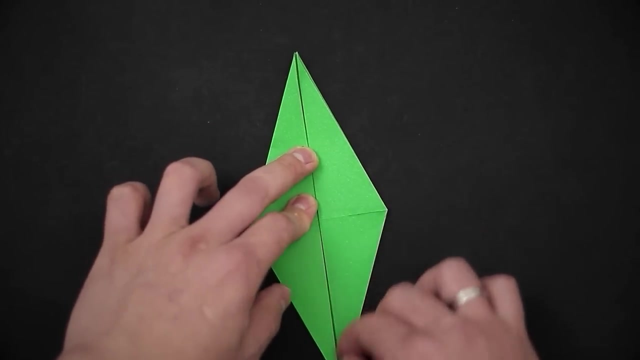 Okay, First we'll bring the edges to the middle, Then we unfold it, Open the first layer and affirm, And, using the lines that we made, let's bring both sides to the middle. This is the result. Keeping this position, let's fold a new diagonal on the right side. 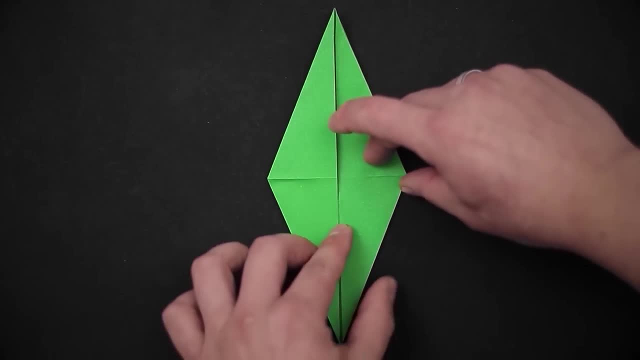 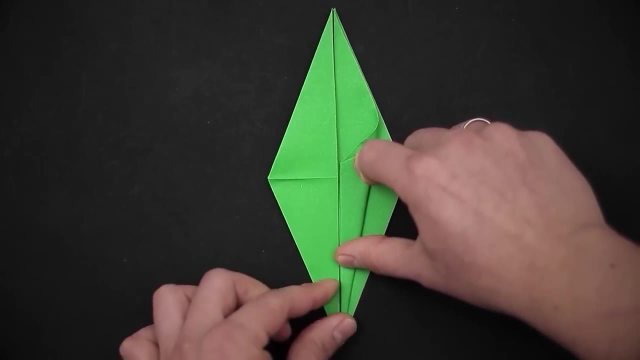 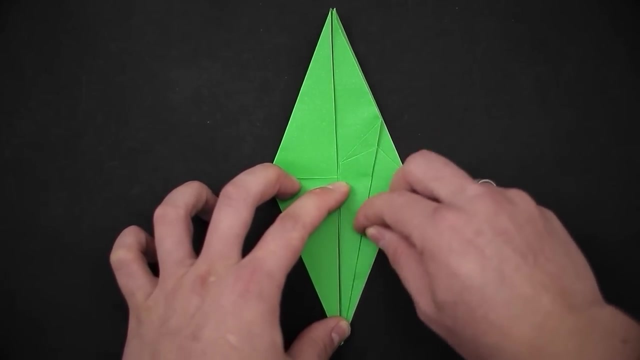 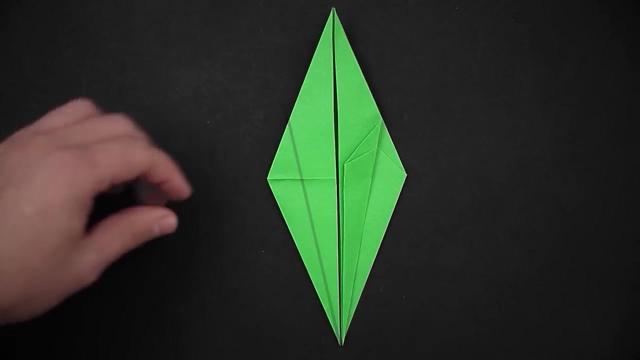 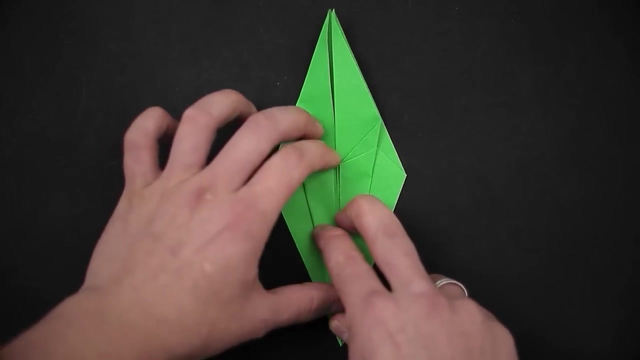 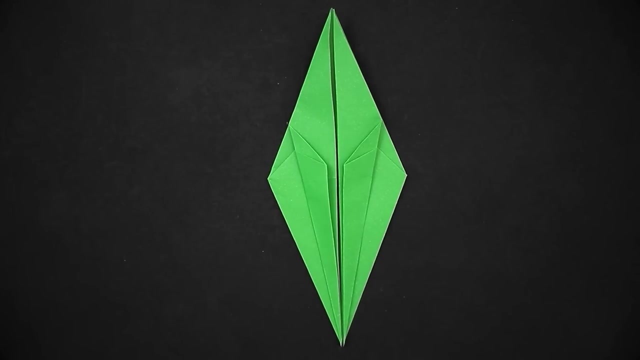 Just like before, we'll have to bring the diagonal edge to the middle And reinforce. The right side is ready. Let's fold the same diagonal on the left And repeat the same thing on the other side. Having done that, let's turn the paper over. 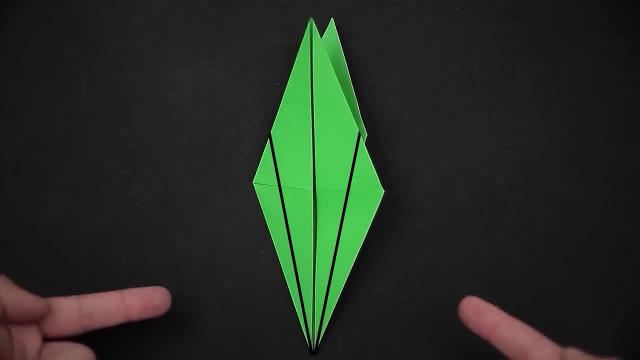 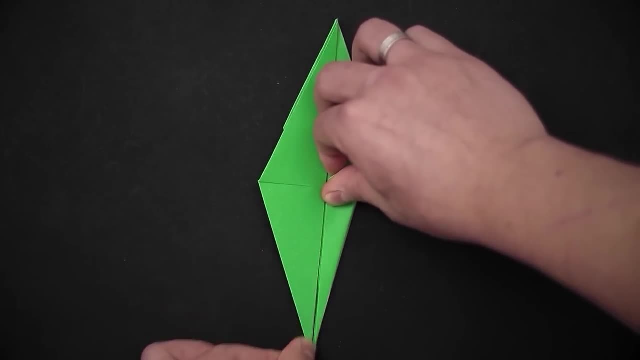 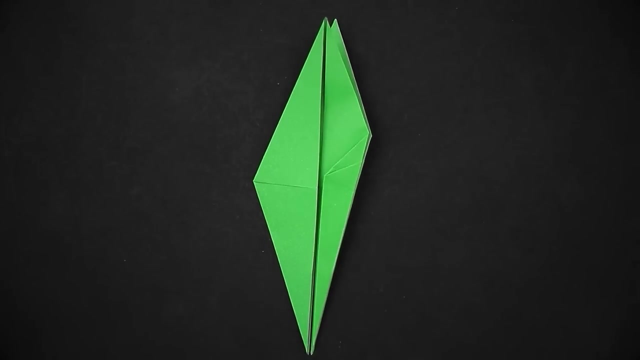 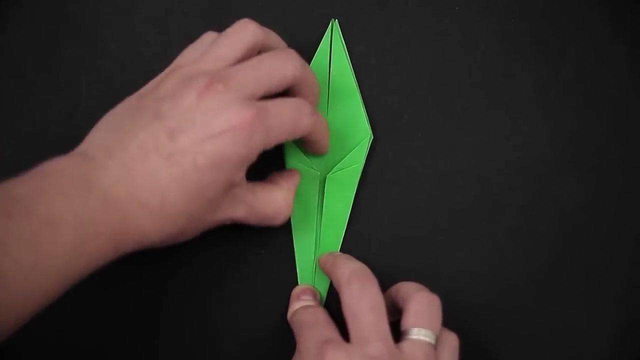 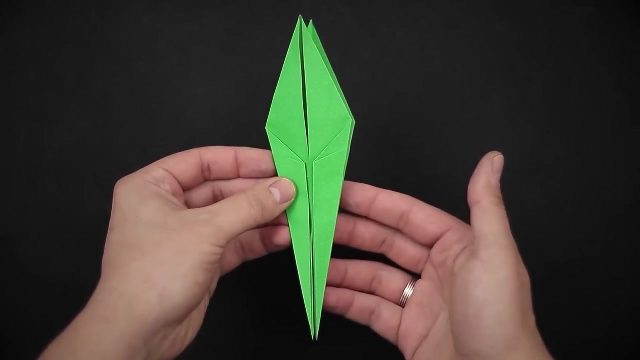 And repeat the same thing here on the other side, First the right side to the middle, And then the left side to the middle as well. From now on, we're going to make the details of the dragon, So let's open the right side like this: 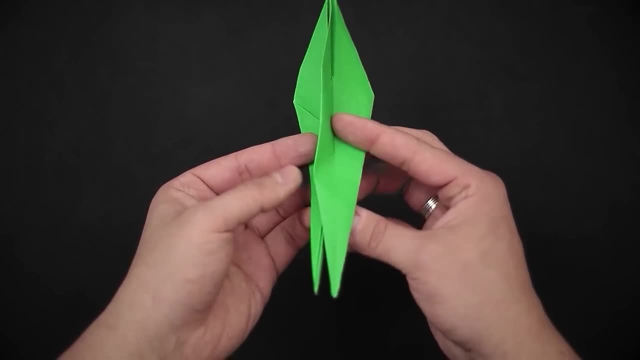 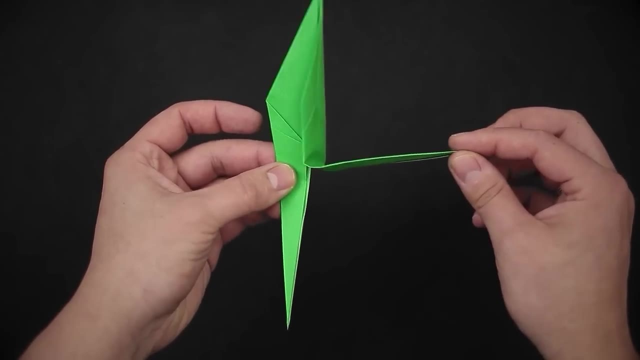 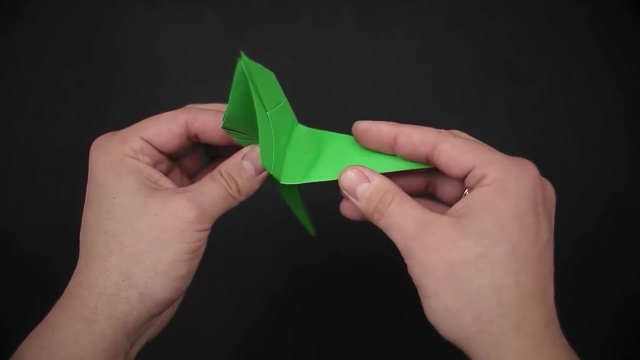 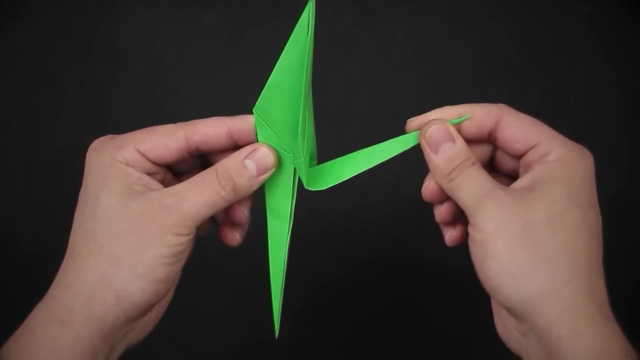 Then we're going to bring this part to the side. Next, let's close the same part by bringing the middle crease up. Basically, we just reversed the paper. Now we're going to close the right side again, But now over this part, we just reversed. 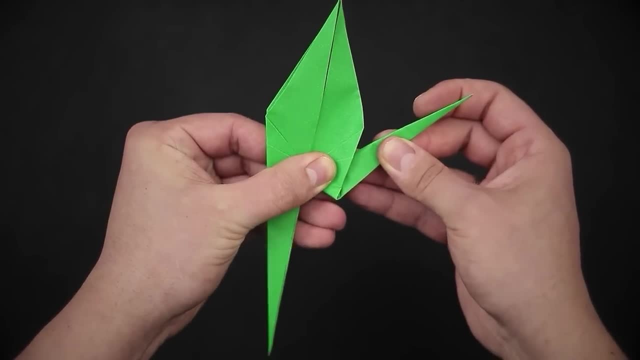 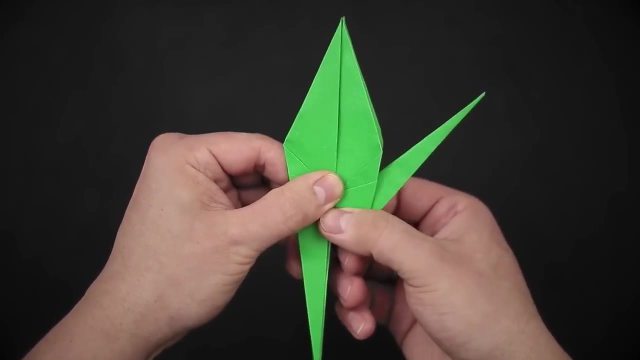 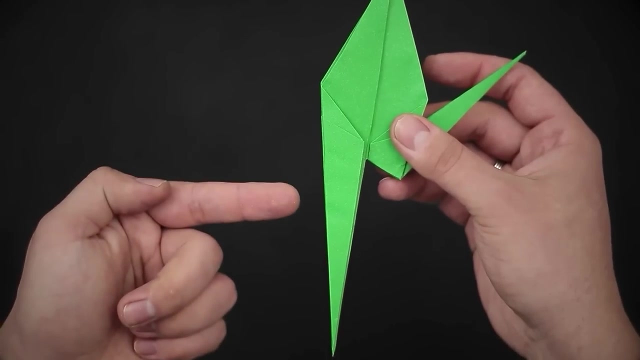 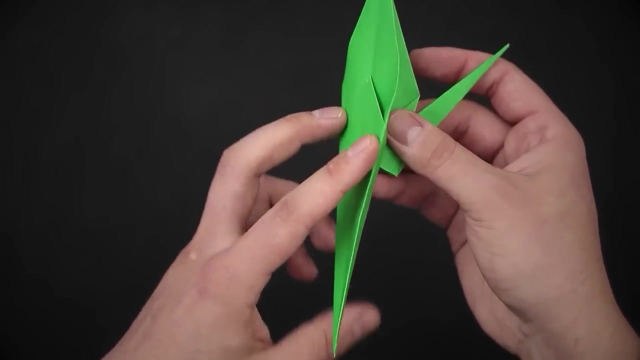 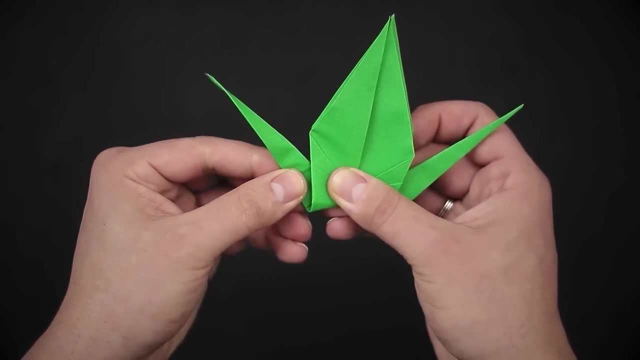 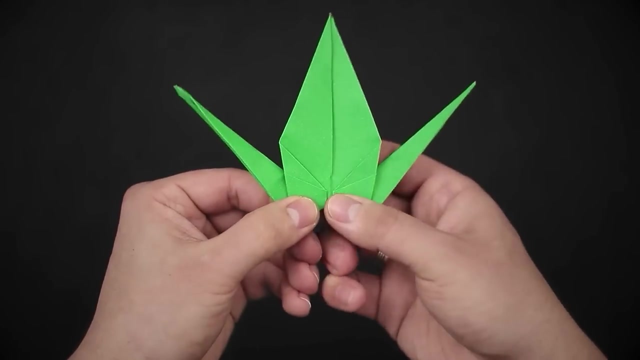 This fold needs to be about this angle here, But you can change it a bit if you want. Now we just need to repeat the same thing here on the other side, Leaving the fold at the same height, And then we fold back, Then we fold these larger flaps down. 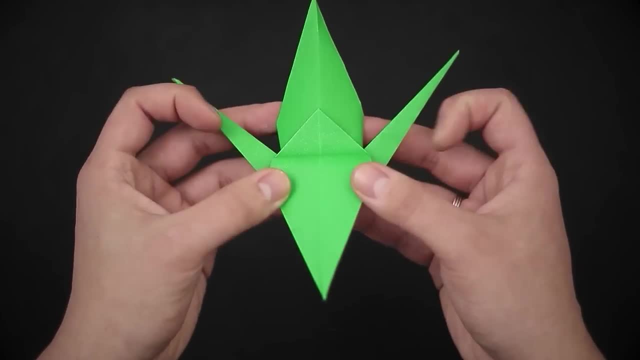 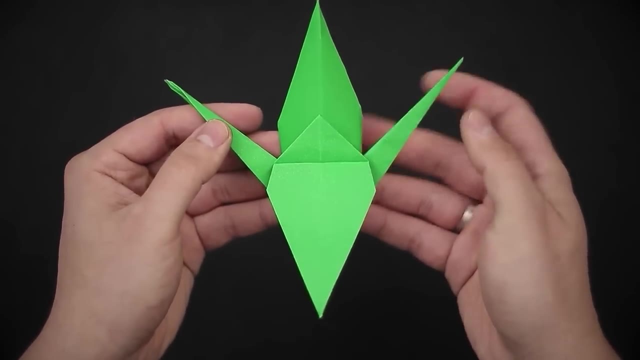 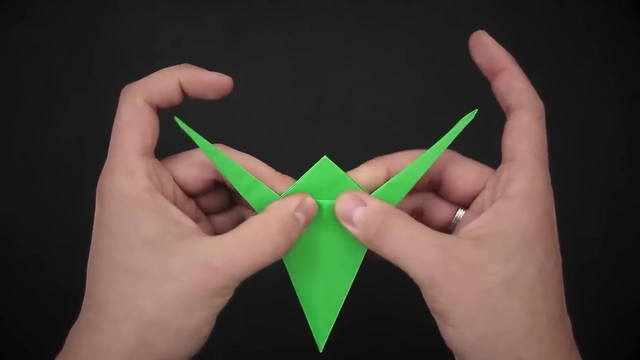 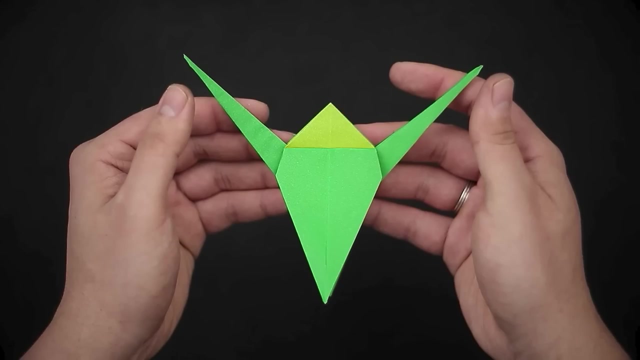 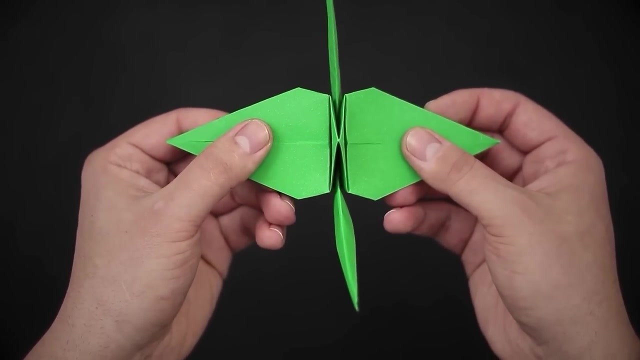 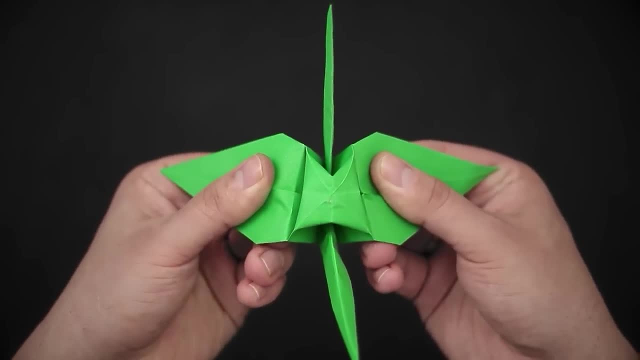 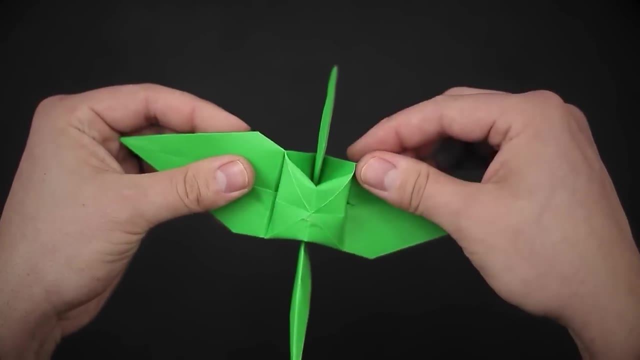 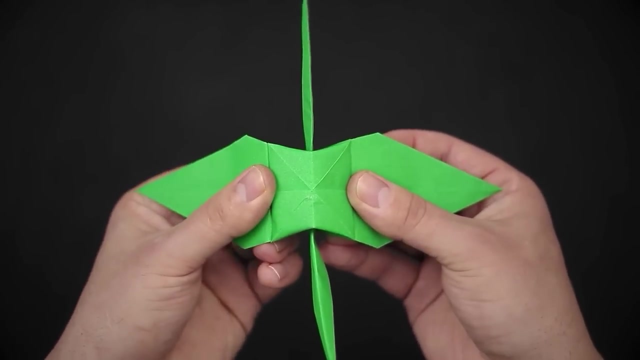 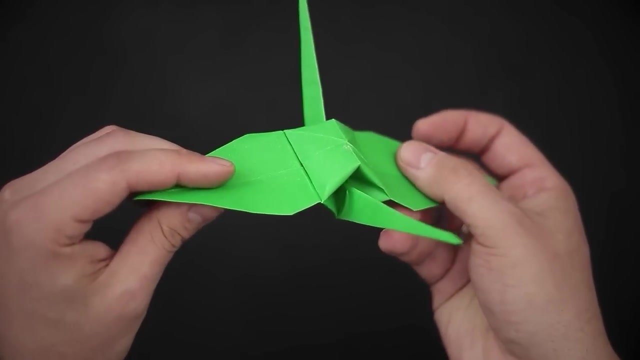 causing this same triangle to inflate, to open like this. The middle part will be easier, but the corners will take a little more work, so I recommend you to be very careful. Once we have this part open, we're going to have to close it again, but this time in a 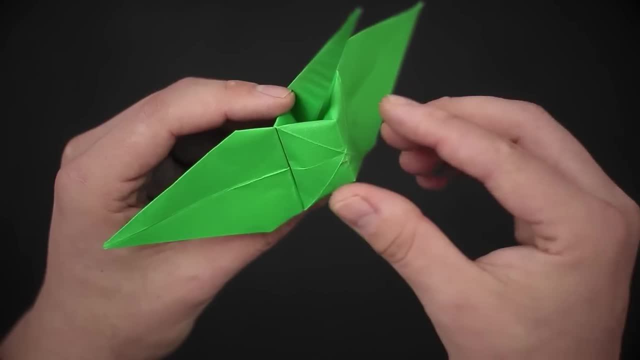 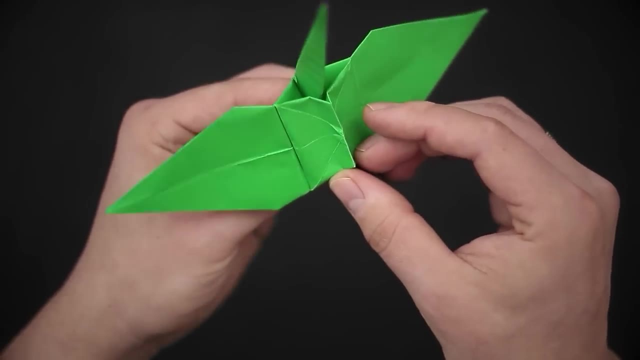 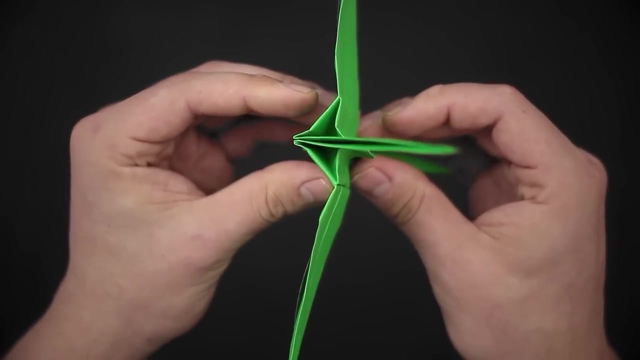 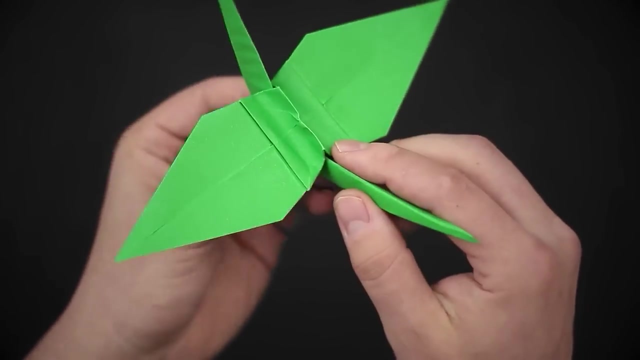 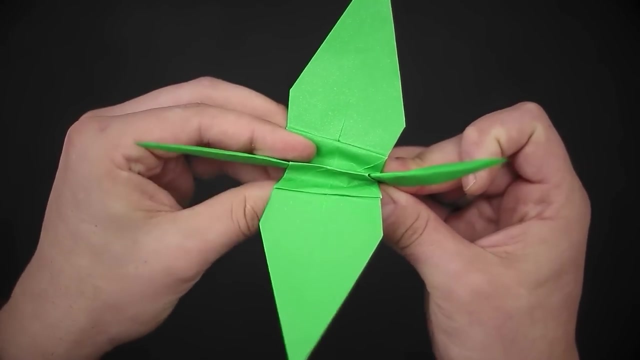 way that only the middle part is on top. To do that, just pinch the paper like this and push the sides towards the middle. It will more or less get the correct shape automatically. Just watch and try to repeat the same. 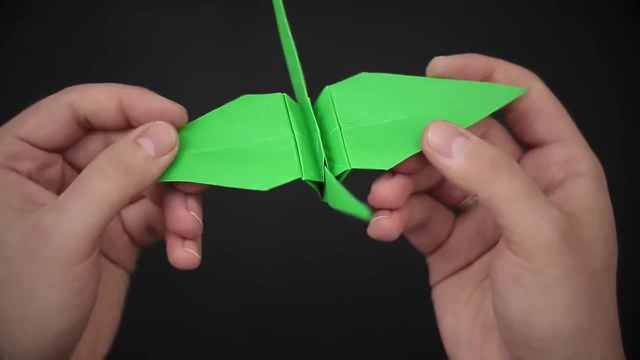 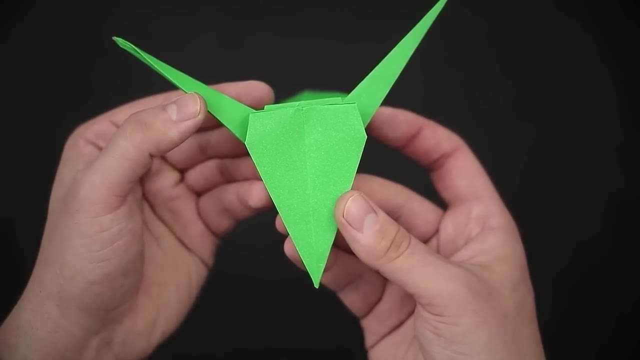 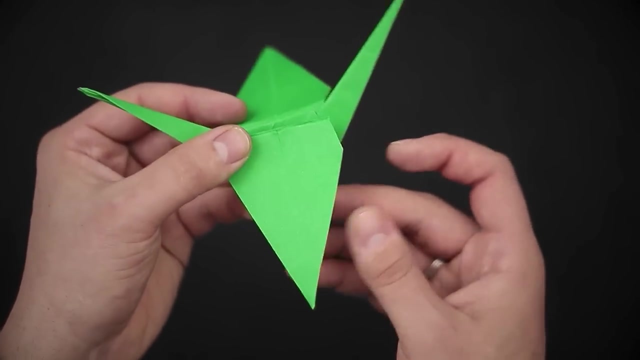 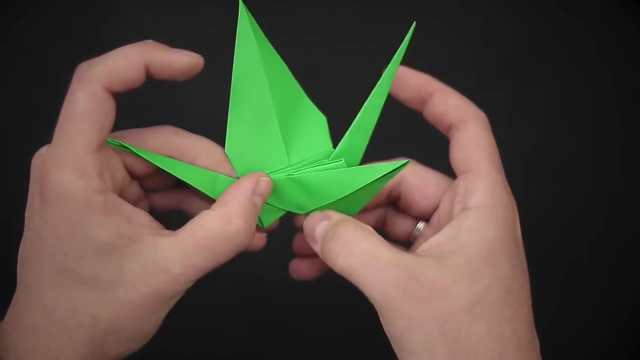 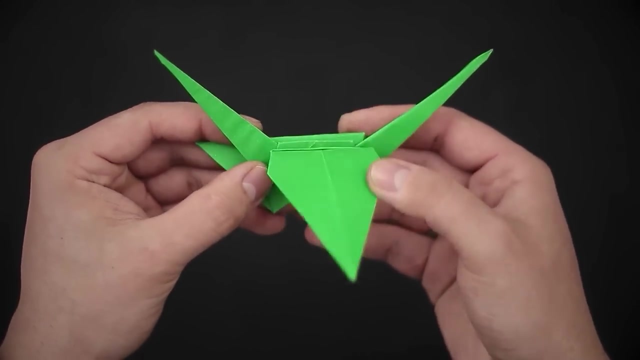 This will give us a nice detail on the back. Now let's make the wings. Let's take one of these larger flaps and fold the diagonal edge to the horizontal just above. Let's turn it over. Repeat the same thing with the other. 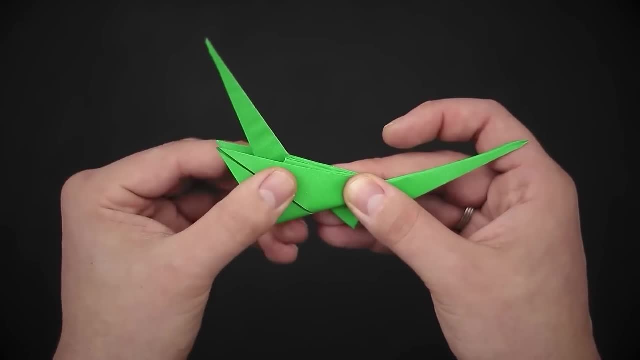 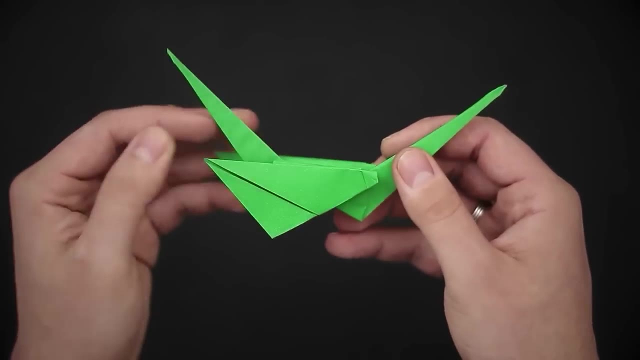 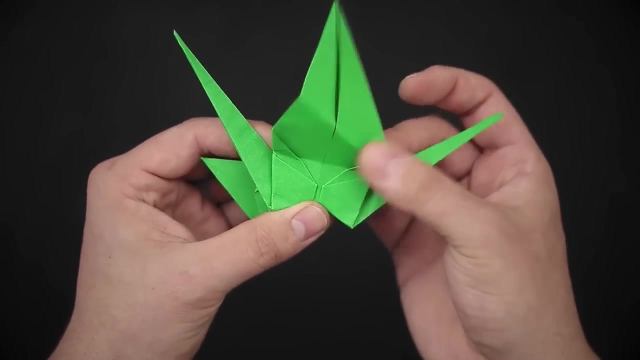 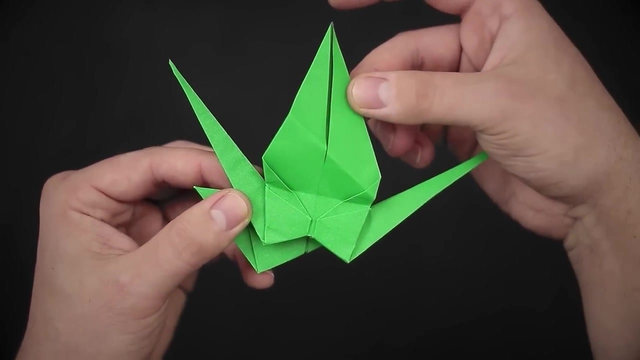 And now we can unfold this. The wing was divided into two. For the next step, we're going to take the bottom part and fold it in half. And now we can unfold this. The wing was divided into two. For the next step, we're going to take the bottom part and fold it in half. 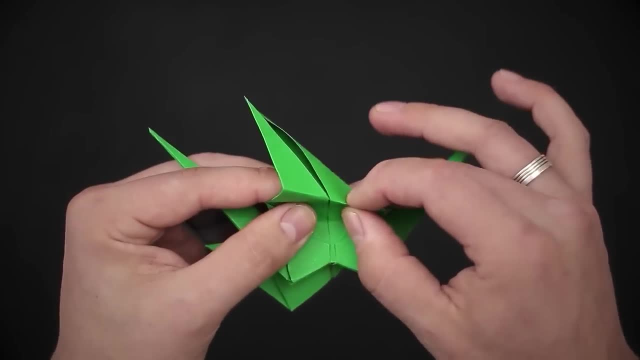 And now we can unfold this. The wing was divided into two. For the next step, we're going to take the bottom part and fold it in half. And now we can unfold this. The wing was divided into two. For the next step, we're going to take the bottom part and fold it in half. 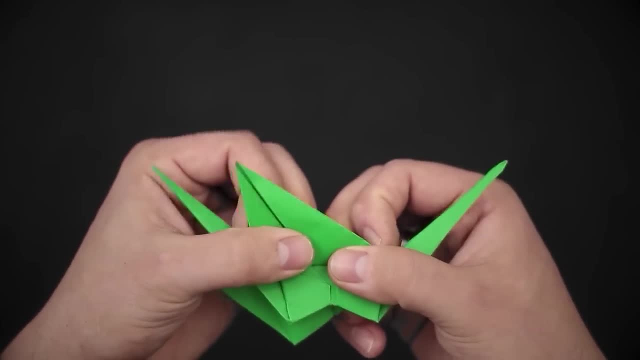 And now we can unfold this. The wing was divided into two. For the next step, we're going to take the bottom part and fold it in half. And now we can unfold this. The wing was divided into two. For the next step, we're going to take the bottom part and fold it in half. 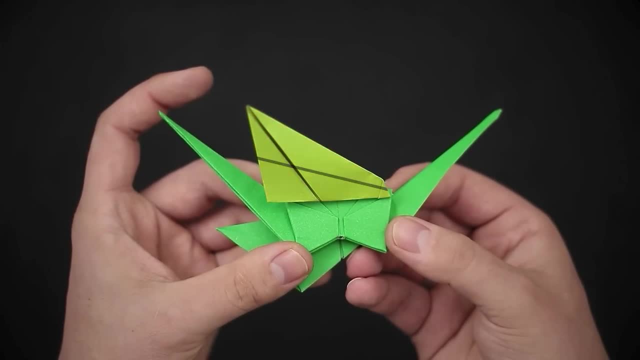 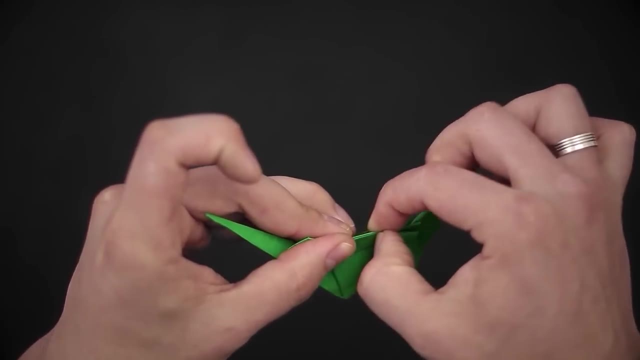 And now we can unfold this. The wing was divided into two. For the next step, we're going to take the bottom part and fold it in half, And now we can unfold this. The wing was divided into two. Now the first wing is ready. 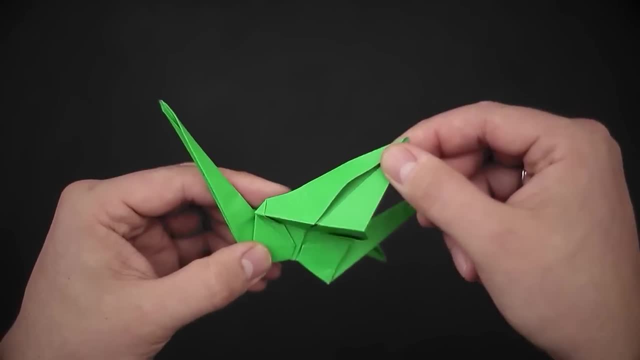 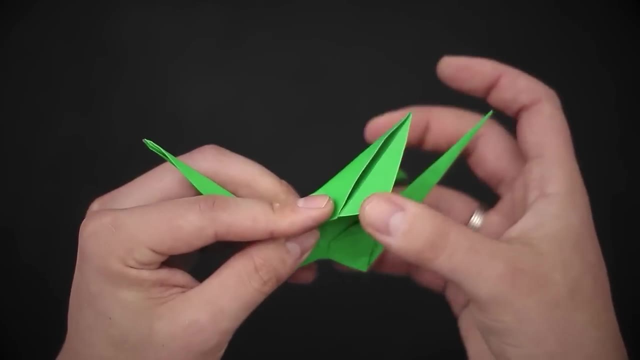 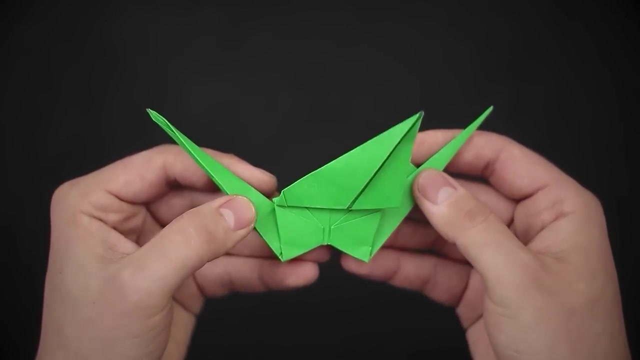 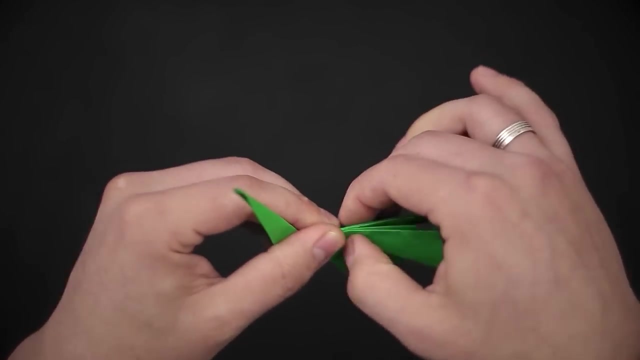 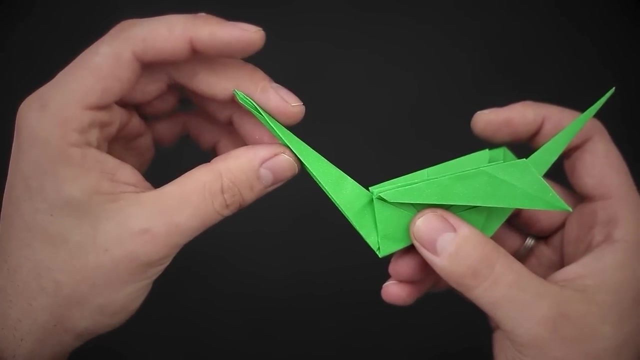 Let's go to the other side and repeat the same thing with the other. First we fold the bottom half And then the top half. To make the head is very simple. We just need to open this end here in the front, Reverse it down. 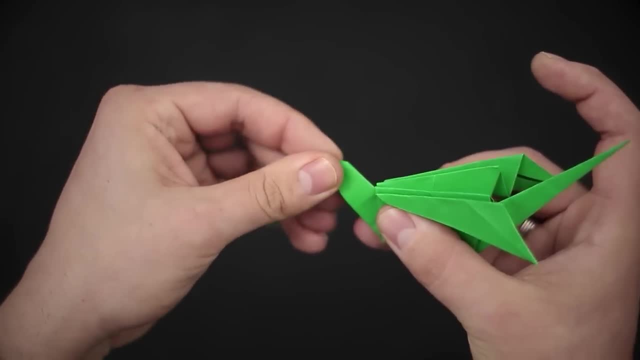 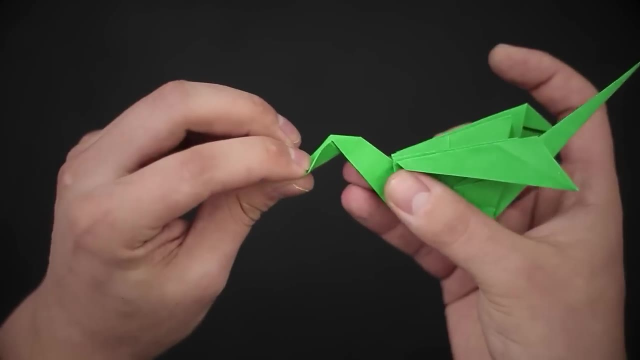 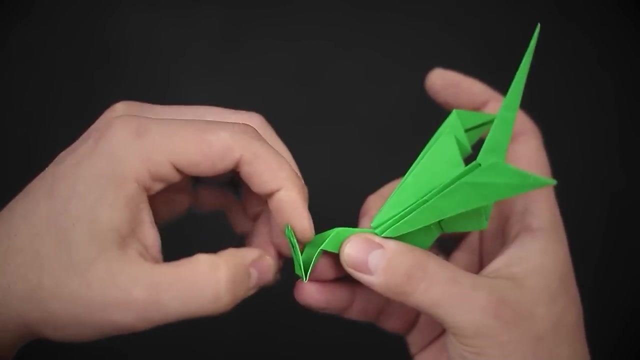 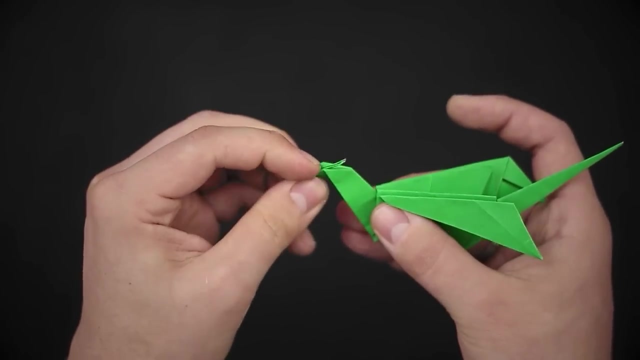 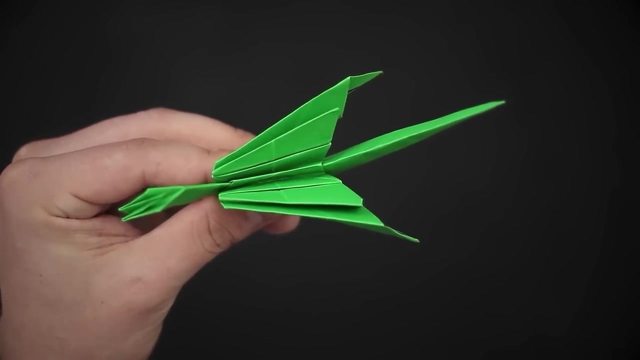 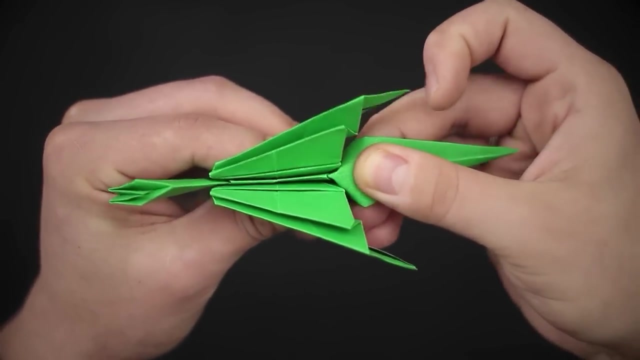 Folding it more or less in half. Then we'll fold it back up. Now that we have the head part ready For the tail, You can make it the variation you want, But I think it's really cool to open the tail like this.